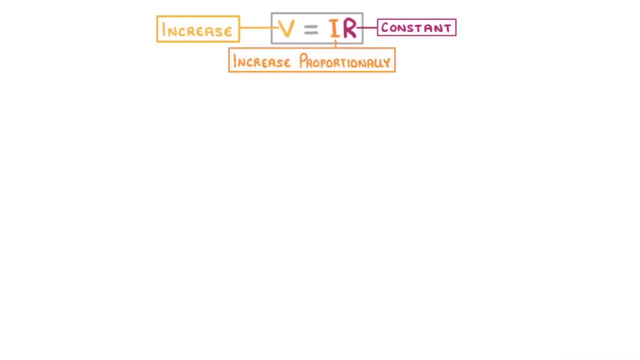 should increase proportionally or vice versa, And we can see this if we plot a graph of current against potential difference. As the potential difference increases, for example, we use a bigger battery, The current produced in the circuit would also increase, And this negative part down here just shows the same thing, except the battery is attached. 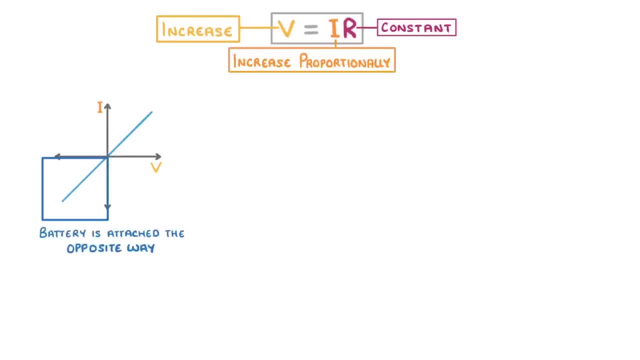 the opposite way around, so the voltage and current are effectively negative. We get these nice straight lines in circuits that contain only wires or resistors, because for these circuits the resistance stays constant the entire time, which, remember, was the requirement we mentioned earlier. 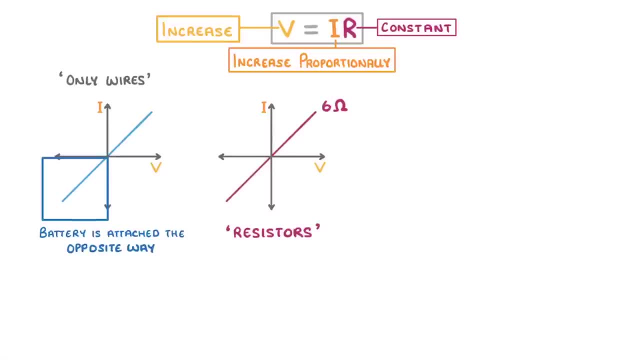 So what are the resistors? If we used a different wire or a different resistor, the line would still be straight, but it would be more or less steep. For example, a bigger resistor would have a less steep line, like this one for a 10 ohm. 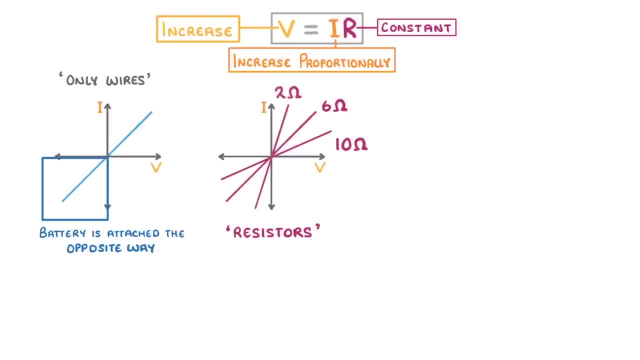 resistor, While a smaller resistor would have a steeper line. You can think of this in terms of how much potential difference is required to produce a given current. If the circuit contains a smaller resistor and so less overall resistance, then we only need a small potential difference to drive a large current. 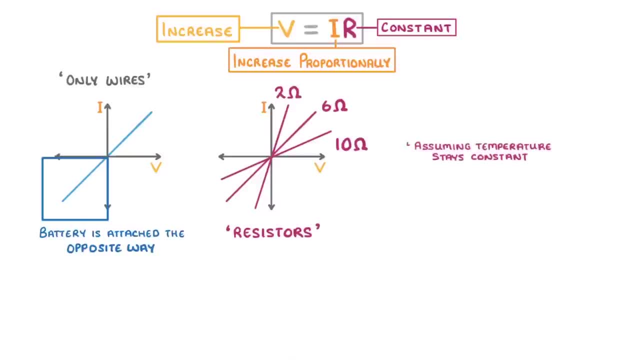 One thing to mention here is that we're assuming that the temperature stays constant. If we increased the temperature, then the resistance would also increase, And in reality, higher currents do generally cause wires to heat up if they're left on for a while. 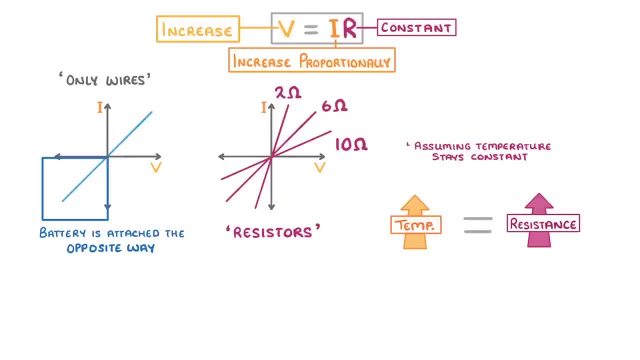 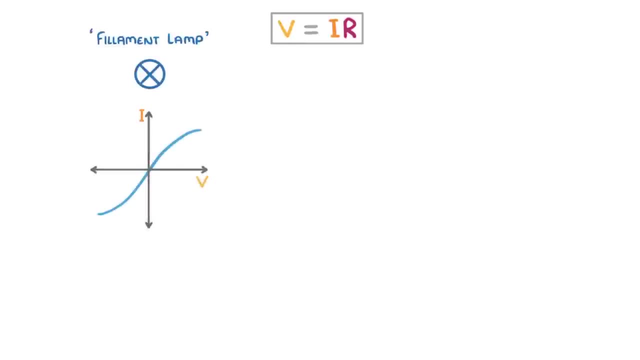 So in practice, the lines don't always look quite this straight. The next thing we need to look at are the graphs of filament lamps and diodes. Filament lamps are just light bulbs which contain a very thin metal filament, And as the current flows through the filament, the wire heats up until it's so hot that 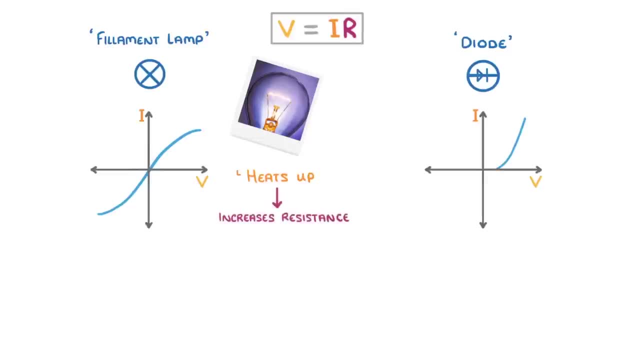 it emits light. All of this heat massively increases the resistance, though, and so the curve gets less steep as we increase the current, Which is just showing that less current can flow per unit of potential difference as these higher voltages do, because the temperature and resistance is so much higher.